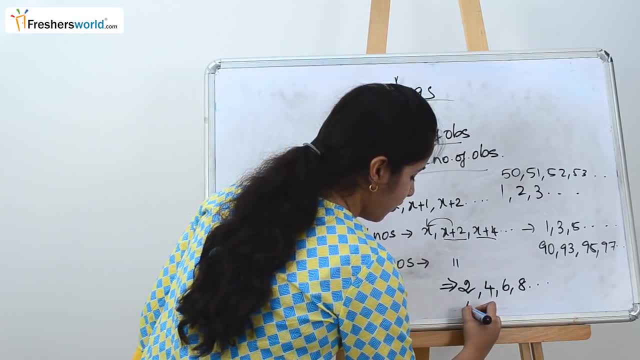 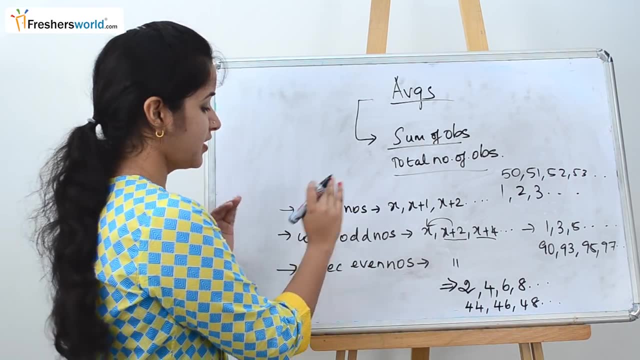 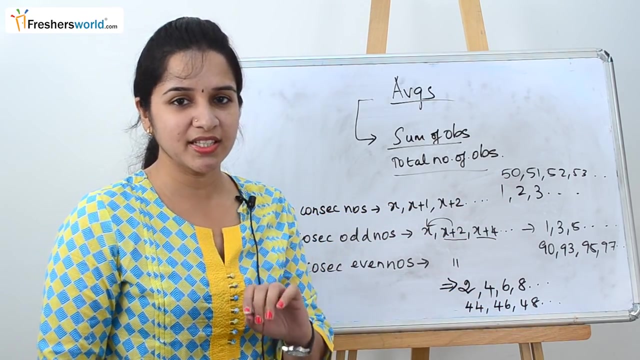 Let's take- I am taking- the x is as 44. So it becomes 44,, 46,, 48 and so on. So now you understand the concept of consecutive numbers, consecutive odd numbers and consecutive even numbers. When you face these type of questions, I will tell you how easily to find the averages of them. 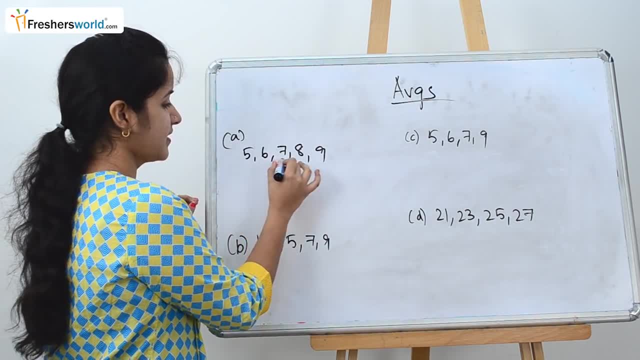 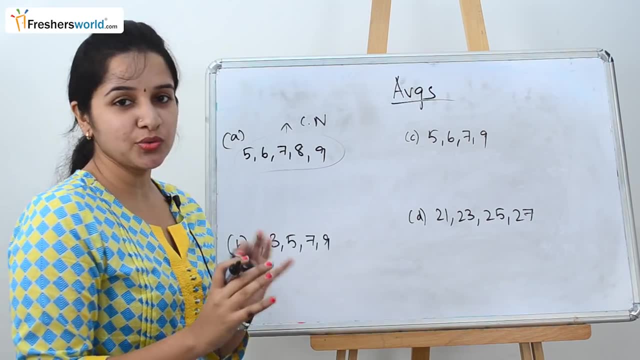 So first question that they have given is 5,, 6,, 7,, 8,, 9.. So, as you can see this, these are consecutive numbers. So by seeing this, you don't have to do the general averages formula like adding all these, dividing it by 5.. 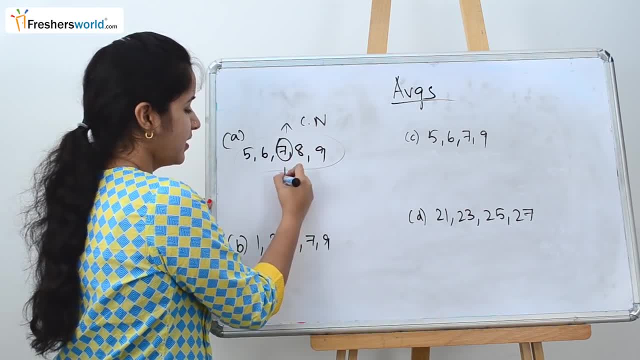 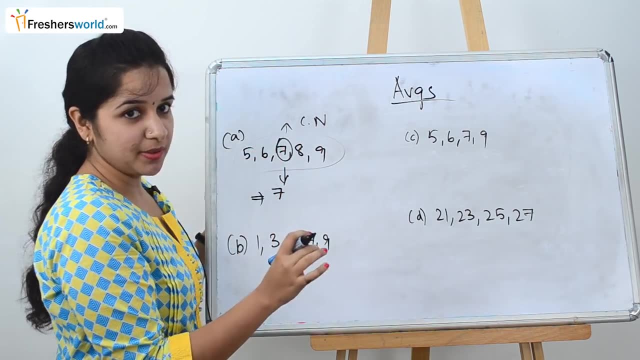 By seeing this. it is always known that the middle number is your average. You can cross check it by adding it and dividing it by 5. So if you are given a consecutive number, always remember that the middle one is the answer for that. 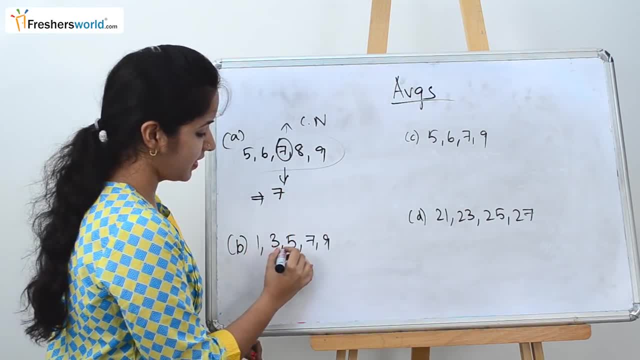 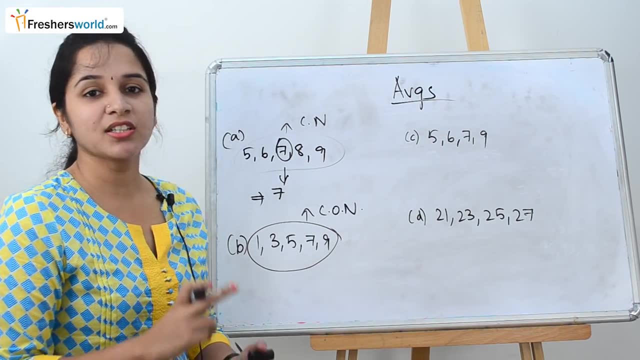 Let's take another example. What is the question here? 1, 3,, 5, 7.. So this is nothing but consecutive odd numbers. So similarly, let's take it for consecutive odd numbers or consecutive even numbers, or whatever be the question. 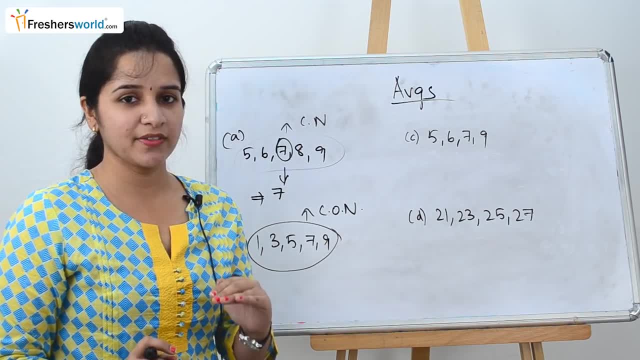 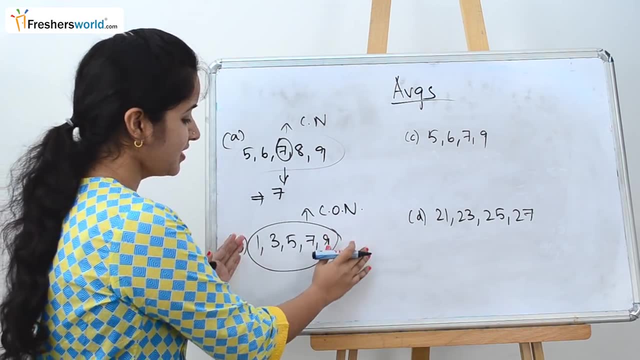 Why we understood the consecutive numbers, consecutive odd and even numbers. That's because all these three types, always the middle number will be your average. You should always remember this. Once you see this, you don't have to calculate anything. Within split second you can write: the average is nothing but 5 here. 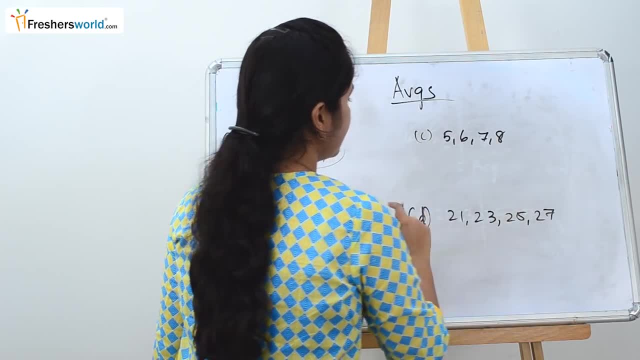 Let's take the next question. So they have given as 5,, 6,, 7,, 8.. So these are consecutive numbers. So, as we know that in consecutive number we should always take the middle number as average, 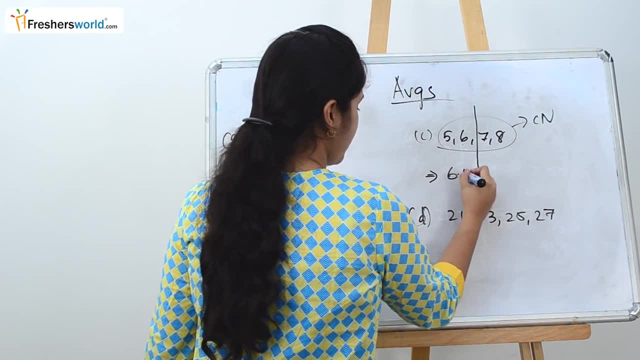 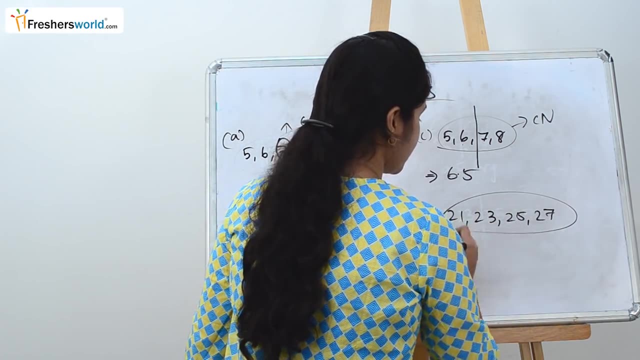 So middle between 6 and 7, which is nothing but 6.5, which is the average. Let's take another example. So what they have given, 21,, 23,, 25,, 27, which is nothing but consecutive odd numbers. 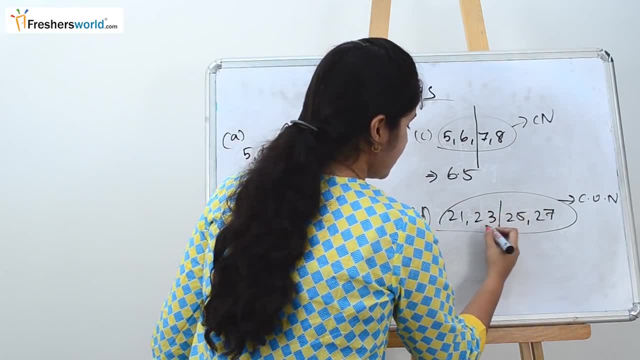 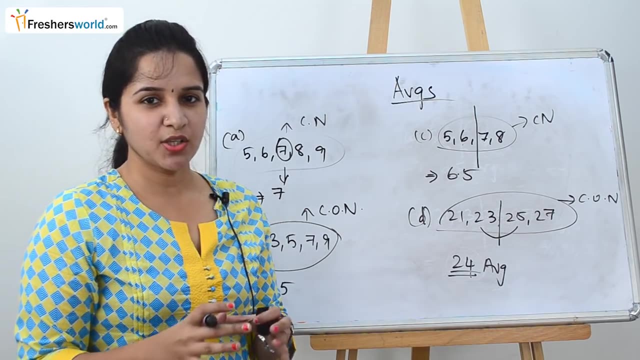 So, as usual, we take the middle number as the average. So what is between 23 and 25?? It's nothing but 24.. So 24 is the average here. So if you see the question to be falling under consecutive numbers, or consecutive odd numbers, or consecutive even numbers, 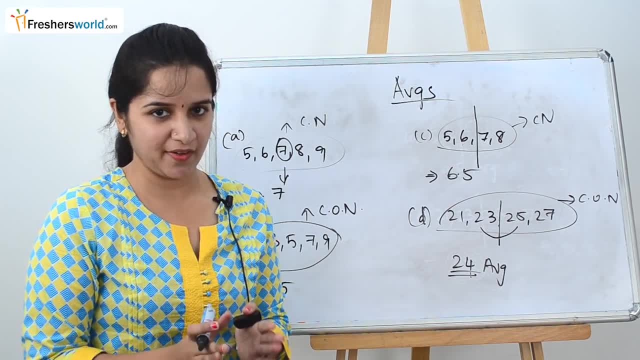 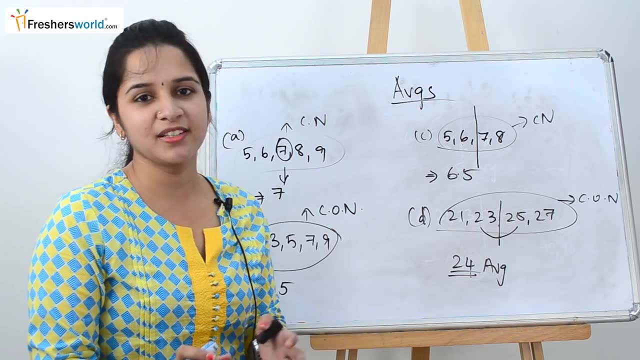 always remember the middle number will always be your average, So you don't have to waste your time in finding out the average formula and doing substitution In split second. as you see the question, just write the middle number as the answer. Let's solve a couple of problems in averages. 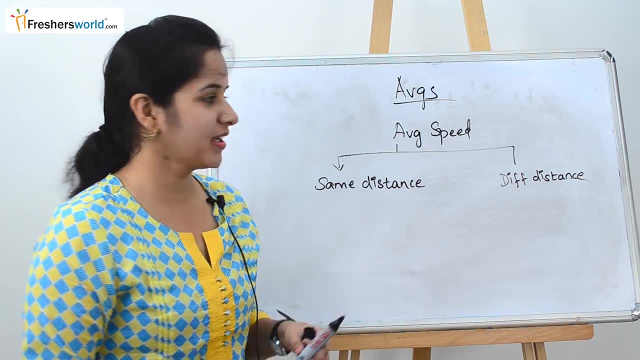 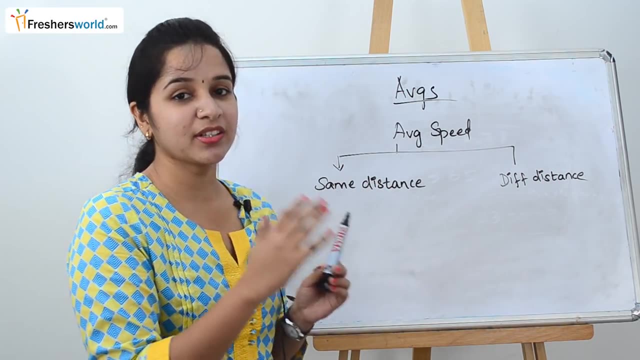 So in case of averages, the common type problem that you see is average speed. In average speed there are two concepts: If they are of the same distance and if they are going on a different distance. So in case of same distance, we will face these two formulas. 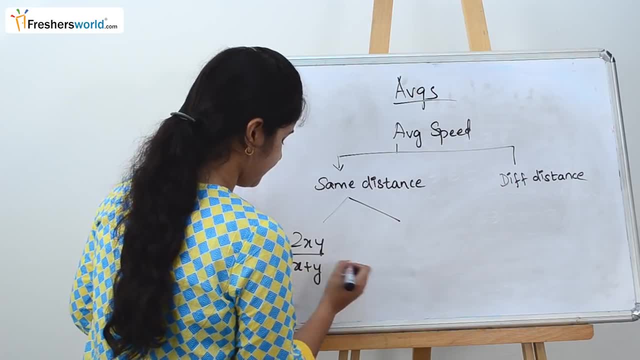 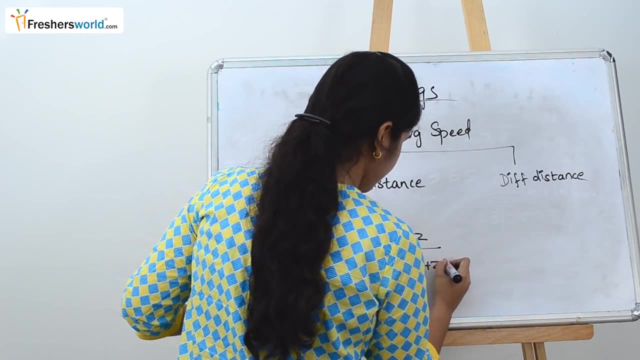 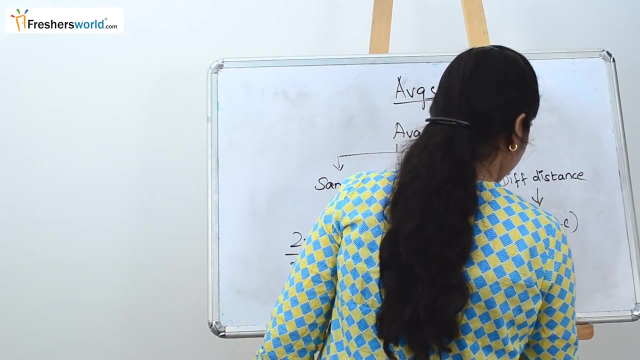 2xy by x plus y, Here 3xyz by xy plus yz plus zx. Similarly, in case of different distance, the formula that we use is a plus b plus c, divided by a by x plus b by y plus c by z. 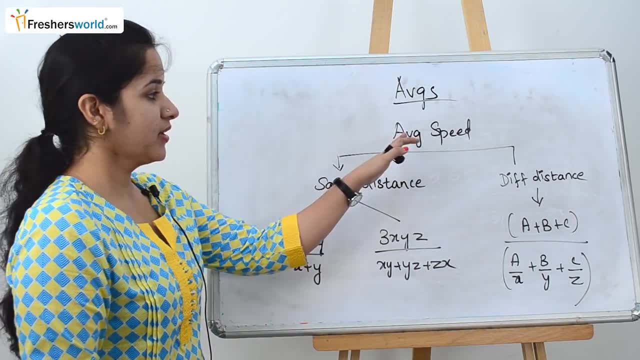 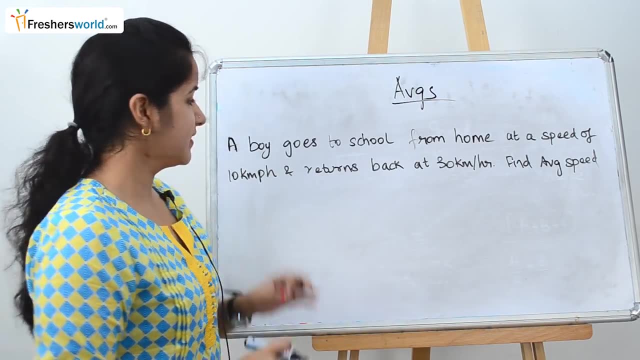 So these are the formulas which we should know for solving the average speed problem. Let's solve a couple of questions to understand this concept much better. The question that they have given is: a boy goes to school from home at a speed of 10 kilometers per hour. 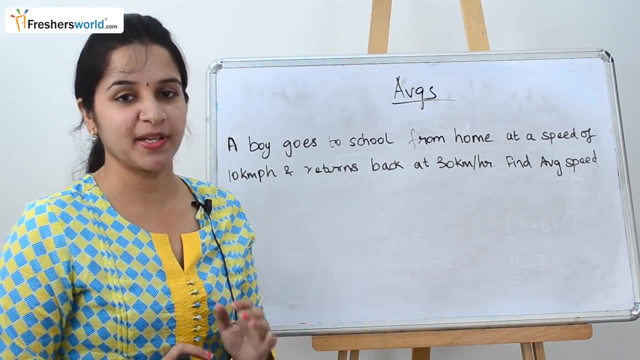 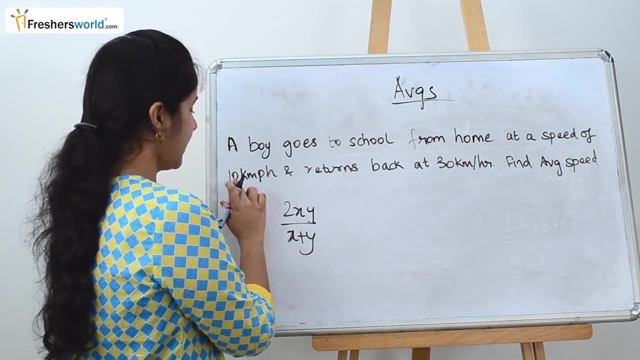 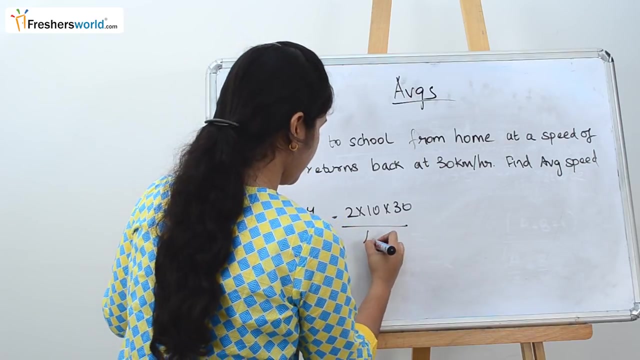 and returns back at 30 kilometers per hour to find the average speed. We know the formula that 2xy by x plus y. Why are we taking this formula? Because they have given two variables like x and y. So 2 into 10, 30 by 10 plus 30 is nothing but 40 here. 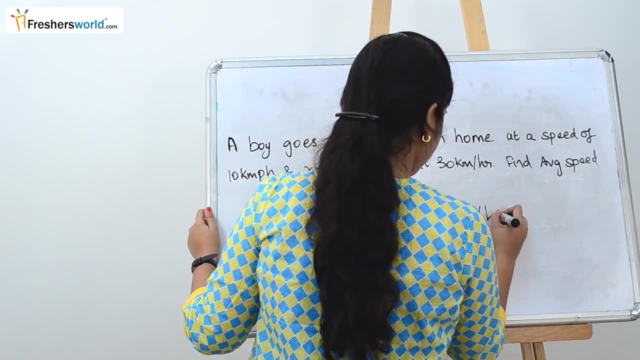 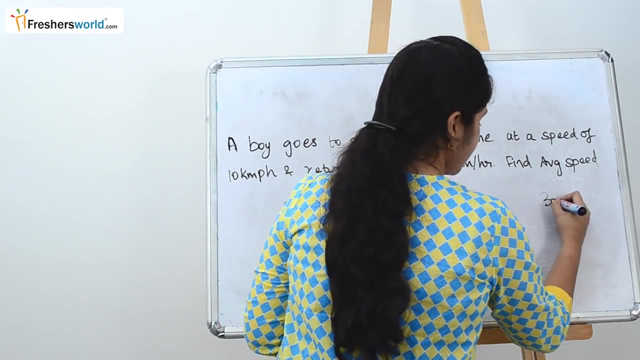 So 15 kilometers per hour is the average speed. How well they can ask. They can give you three speeds and ask you to find it using the formula 3xy by xy plus 30.. 3xyz by xy plus yz plus zx. 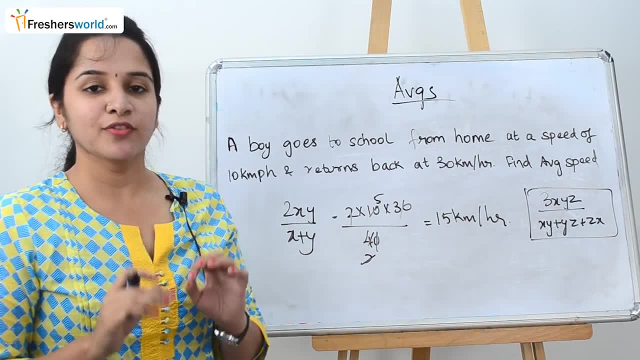 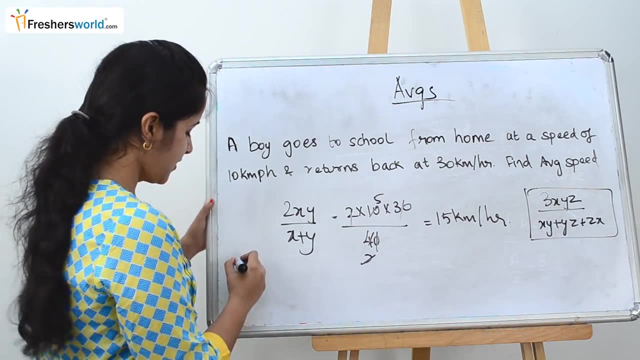 You can substitute in this formula to find the average speed for three variables. What is the other way of asking? They won't give you the speed, They will give you the distance and time. So we know that speed is equal to distance by time. 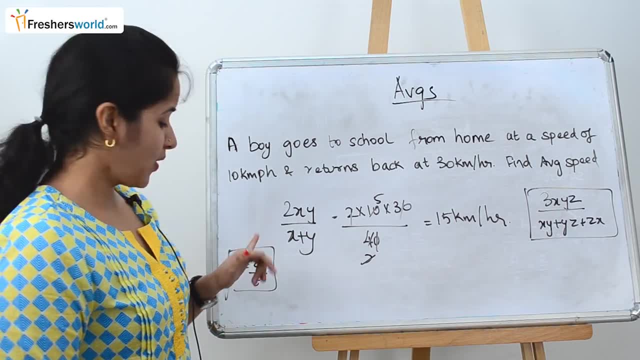 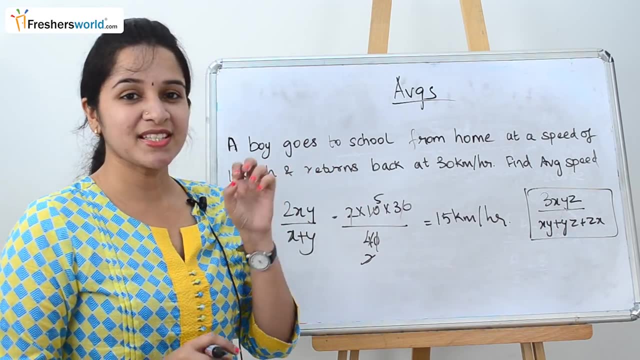 So find the distance by time, You can find the speed. So once you know the speed, you will know the variable And you can substitute in either of the formula. So when you will apply this formula, because it is of the same distance- 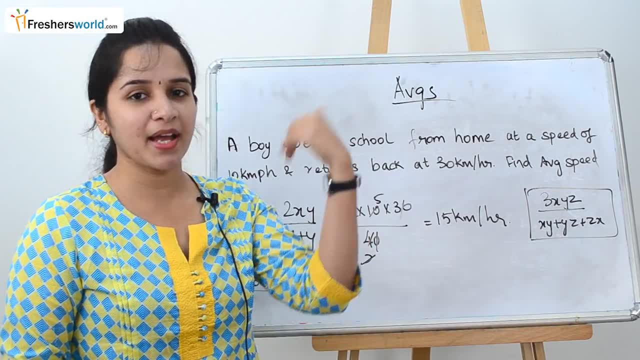 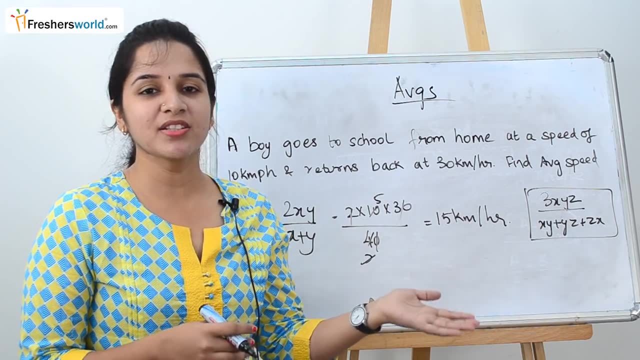 the guy is going to school from home and he is returning back to the home, So he is covering the same distance. Let's take: his distance from home to school is 10 kilometers. Same distance is the one he is going to cover back from school to home. 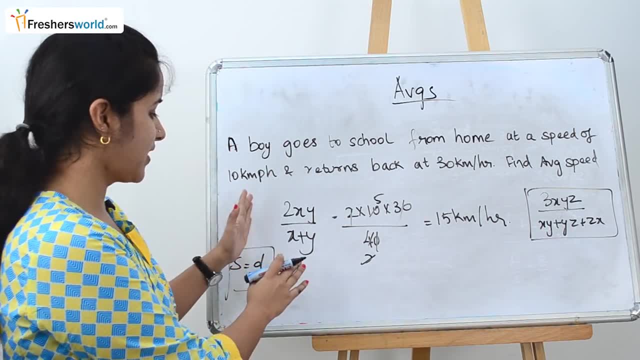 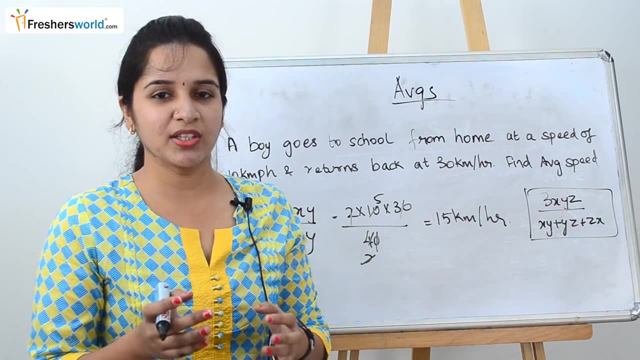 So in case of same distance, we have two formula, which is 2xy by x plus y and 3xyz by xy plus yz plus zx. So let's solve another question with different distance. So in case of this question, 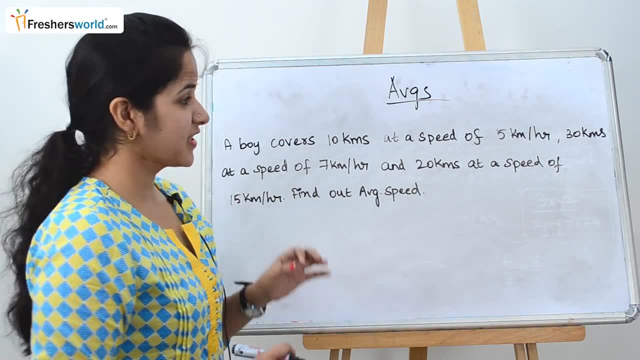 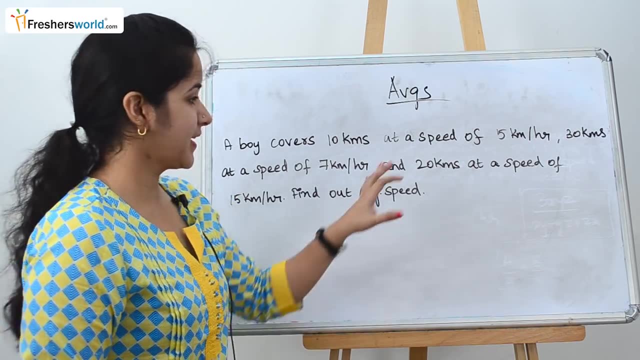 they are giving it, as a boy covers 10 kilometers at a speed of 5 kilometers per hour, 30 kilometers at a speed of 7 kilometers per hour and 20 kilometers at a speed of 15 kilometers per hour. So by seeing the question, we know that he is covering different distances. 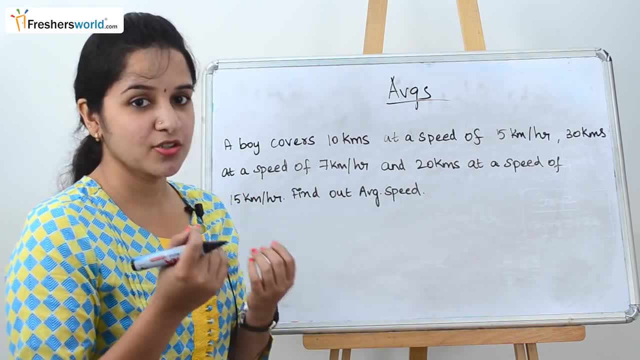 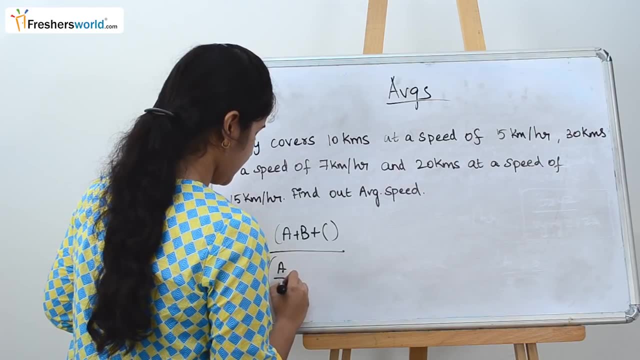 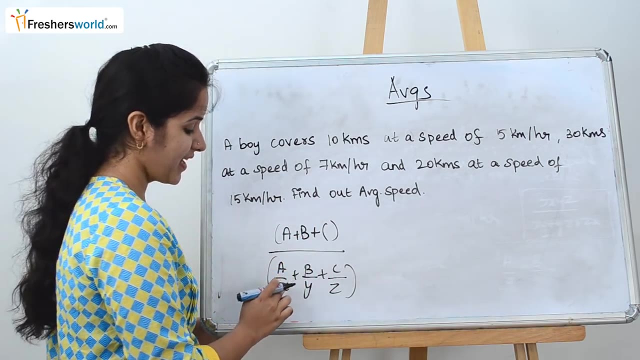 So the formula of different distance will be used here. So what is the formula? a plus b plus c, divided by a, by x, plus b, by y, plus c, by z. So abc means a distance here and xyz is, as you showed earlier. 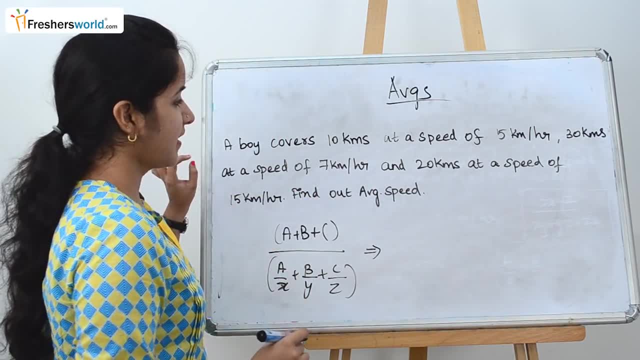 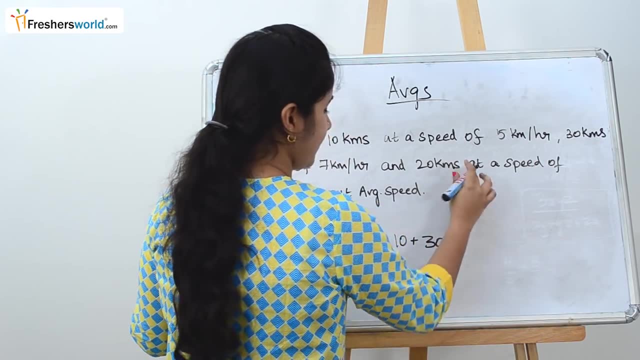 So what is the first distance he is covering? He is covering 10 kilometers, So 10.. Then he is covering 30 kilometers And then he is covering 20 kilometers, So he is covering 10 kilometers in 5 hours. 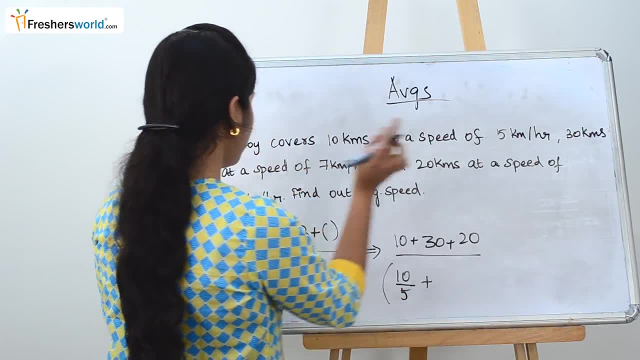 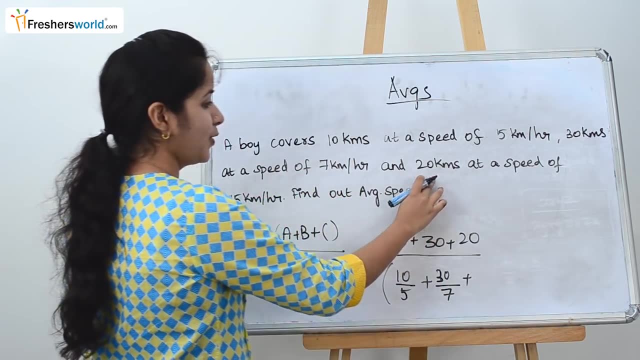 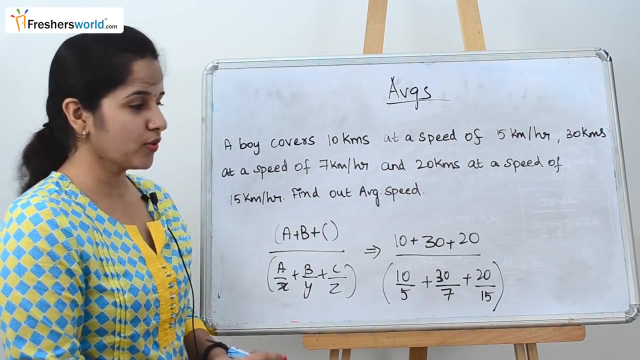 So 10 by 5. He is covering 30 kilometers at 7 hours And he is covering 20 kilometers at a speed of 15.. So once you solve this equation, you will know the average speed that a boy takes for all these distances. 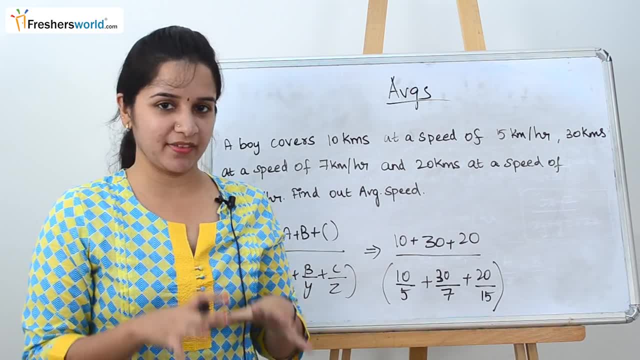 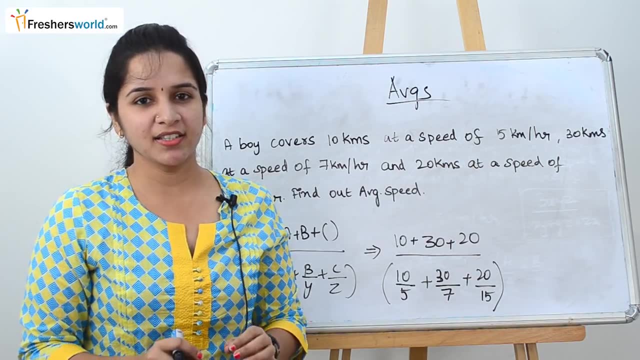 So today we just saw two types of problem in average speed. One is with the same distance and another is with the different distance. These are only the two types of problem that they can ask in average speeds. So if you are a person who is looking for a job, 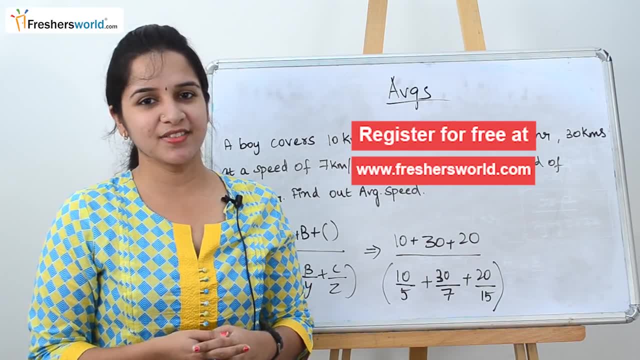 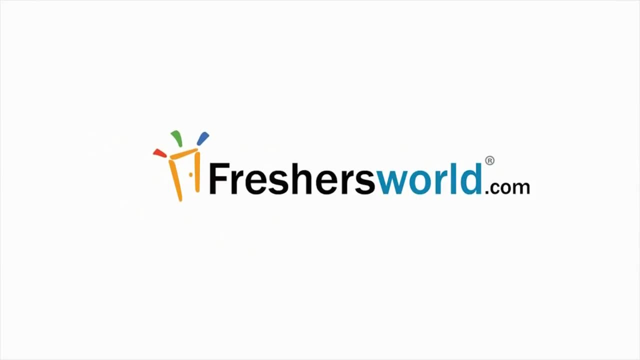 kindly register in our freshersworldcom, Like this video and subscribe to our channel. Thank you, Thank you.